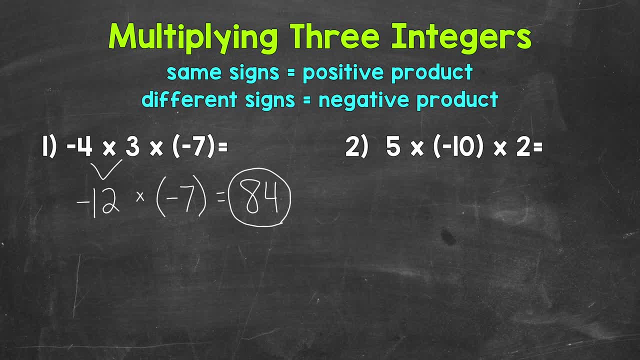 Now I do want to mention one more thing before moving on to number two, and it has to do with the order in which we solved the problem. Since we're only working with multiplication, we can do three times negative seven first and still get the same answer. 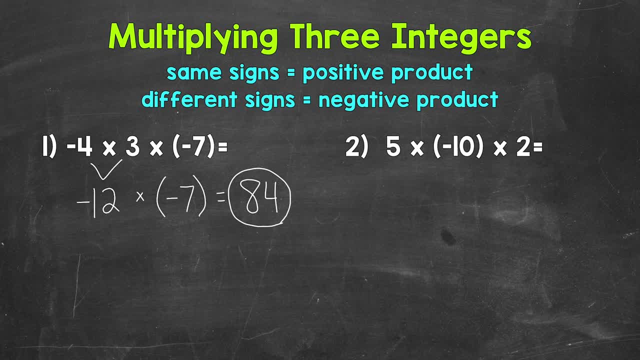 This is because of the associative property. It's how we group our factors. Factors are the numbers we are multiplying. Let's see exactly what that means here. So I will rewrite our problem: Negative four times, and then I'm going to put three times negative seven in parentheses here. 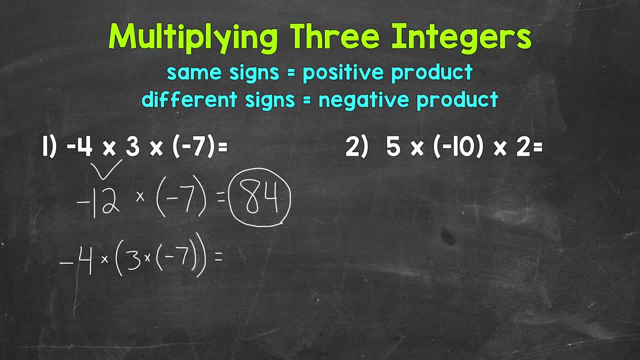 to show that we are doing that first and we are not working from left to right. So three times negative seven, We have a positive, Positive times, a negative, Different signs That's going to give us a negative. Think of this as three times seven, which is twenty-one, and again it's going to be negative. 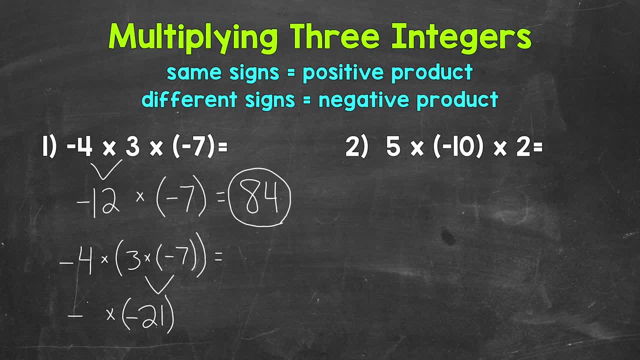 Then we can bring down our multiplication sign and the negative four. So we end with negative four times negative, twenty-one. So we have the same signs, a negative times a negative here That's going to give us a positive. Let's think of this as four times twenty-one. 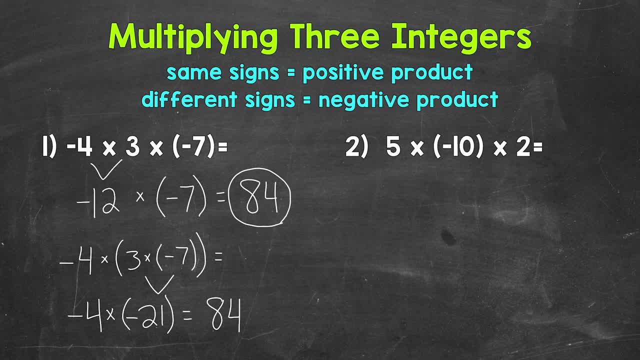 Which is eighty-four, And again it's going to be positive, So we get eighty-four that way as well. So that's something to keep in mind when working through these types of problems. Let's move on to number two, where we have five times negative, ten times two. 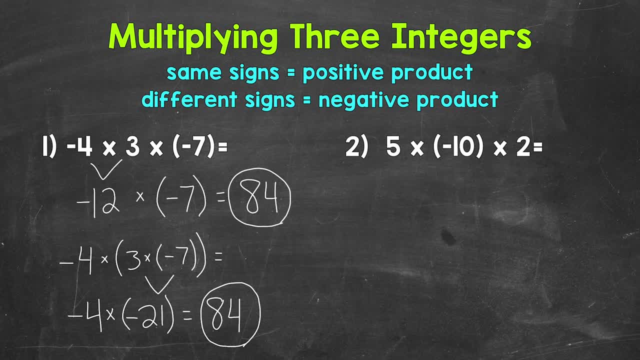 We'll work our way from left to right, starting with five times negative ten. So we have a positive times a negative, Different signs We are going to get a negative. Let's think of this as five times ten, which is fifty. 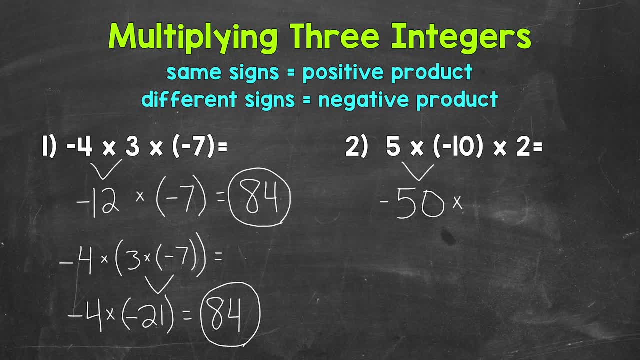 And again it's going to be negative. Bring down our multiplication sign and the two, So we end with negative fifty times two. We have different signs here, a negative times, a positive, so we know it's going to be negative. Think of this as fifty times two, which is one hundred.